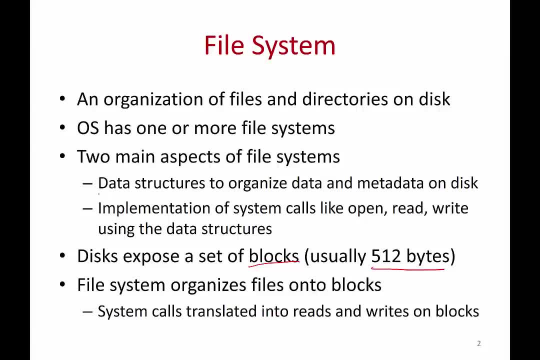 looking at a file system are two things. One is the data structures that are used to organize data and metadata on disk. So the disk contains file data, all the contents of your files. It also has some metadata. right, There is data and there is metadata. What is metadata? It is. 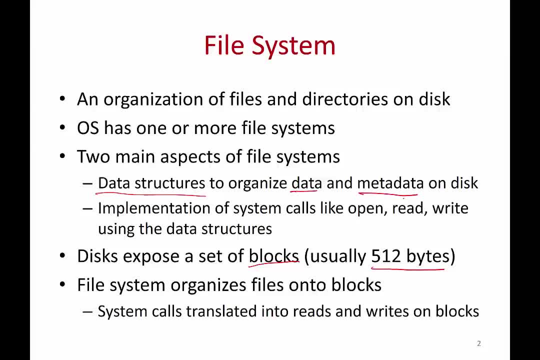 information about the data. For example, what is the size of the file? When was it accessed? All of this is not part of your file data, but it is metadata about the file. So there are several data structures in a file system. to. 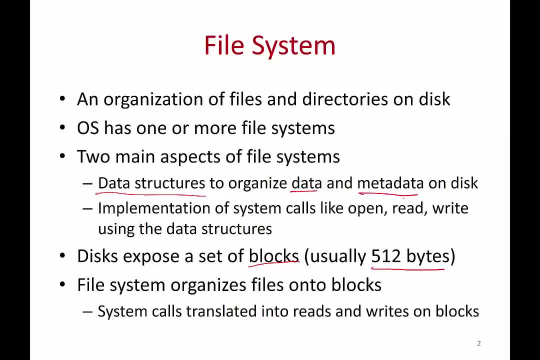 organize all of this data and metadata on the disk. And the next thing to understand when you're studying a file system is to understand the implementation of system calls. So when you open a file, what happens? How are all of these data structures manipulated When you read it from a file, when you 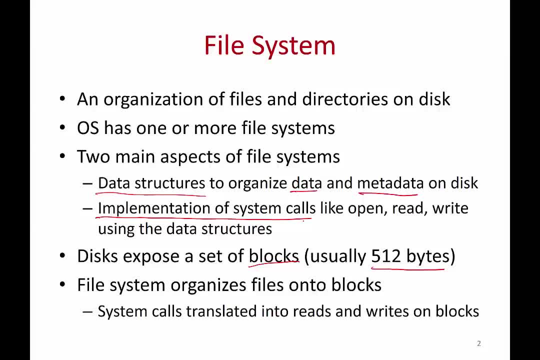 write to a file. So understand the data structures and how system calls are implemented using these data structures, right? Different file systems differ in these details, So when you're looking at a file system, you have to understand the file structure. So in this lecture we want to take an example of a very simple 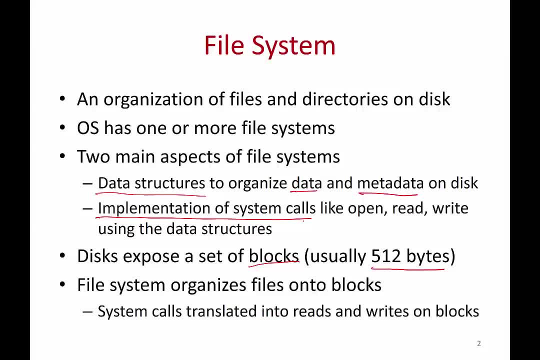 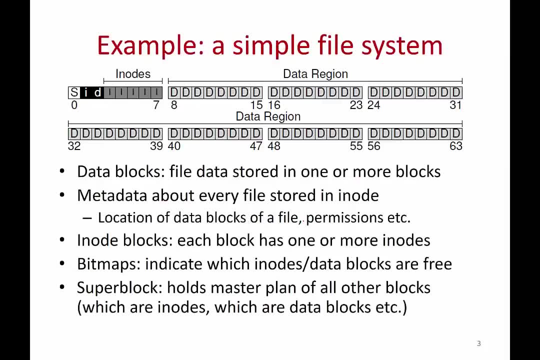 file system to understand the concept of file systems. But you can later read up on more complex, realistic file systems. So let's take an example of a simple file system. Suppose you have a disk with 64 blocks. Here is how the file. 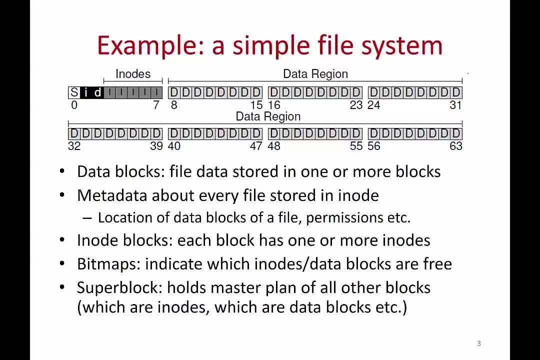 system could organize the disk. Of course, a big chunk of it is the data region right. A whole bunch of blocks are allocated to store file data right. So these are all data blocks and this is the biggest part of any file system. 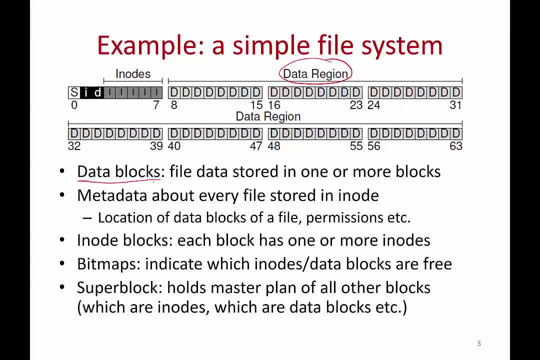 because, of course, this is the most important thing. And then information about every file: metadata, whatever file is stored in an inode, right? So the? what are all the things that an inode has? An inode has things like. here are the: 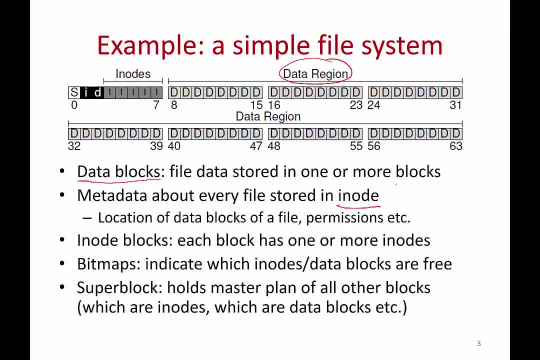 data blocks of the file. Here is the permissions of the file. This is when the file was last accessed. All of that is stored in an inode, And these inodes are stored in set of blocks on the disk, called the inode blocks. right, that's here. so you have data blocks and you. 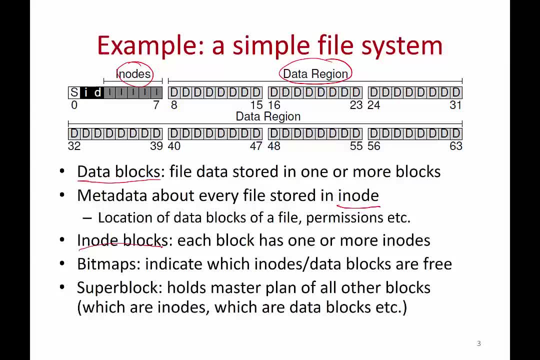 have inode blocks, where each block has one or more inodes and each inode has information about a particular file. and the next thing is: after inode blocks, you have certain bitmaps right which are shown here: this i and d blocks. here are bitmaps, that is, of all of these data blocks, and 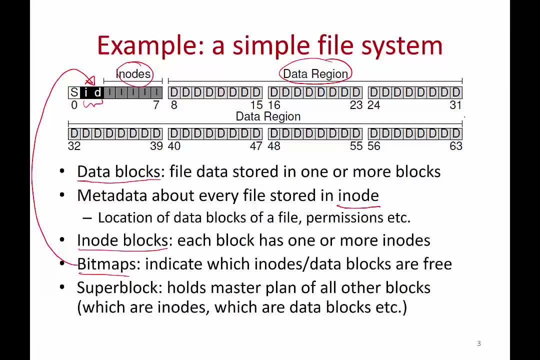 inode blocks. you need some way of tracking which are the free ones and which are the filled ones, right? if i want to create a new file, i should know which data blocks are free, which inodes are free, right? so then you have a set of bitmaps that indicate which of these blocks are free and 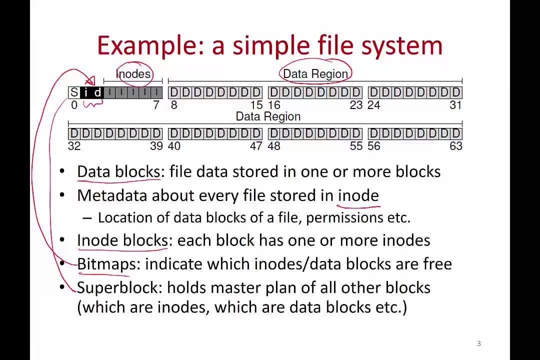 finally, the first block of any file system is the super block. right, what is the super block? the super block basically holds the master plan of all other blocks. the super block says: okay, the next few blocks are the bitmap, the next few blocks, these many blocks- are inode blocks, these many blocks are data blocks. the data blocks are located from. 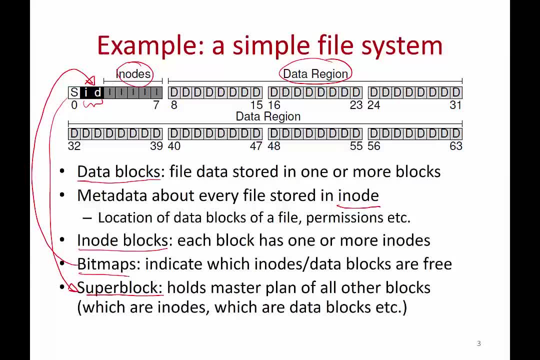 this location to this location. all of that information is stored in the super block, right? so these are some of the main components of the file system organization, right? so a file system takes the blocks in the disk and organizes it amongst these parts. so let's take a. 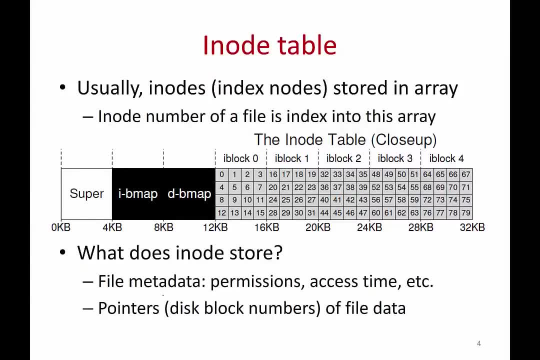 closer. look at the inode table, right? so if you zoom into the initial part of this simple file system, you have the super block, you have the inode bitmap, you have the data block bitmap and then you have the inode table. that is, you have multiple blocks and each block has multiple inodes, right? so you divide the. 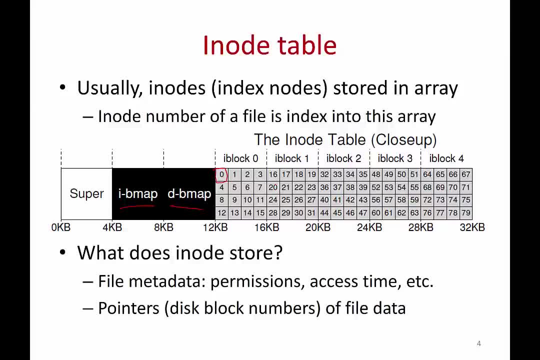 block size. by the inode size you can get how many inodes fit in a block right and every inode have. every file has a unique inode and a unique inode number right. so if a certain file has inode number 41, then you take this array of inodes, you index into inode 41, get this inode and that will have. 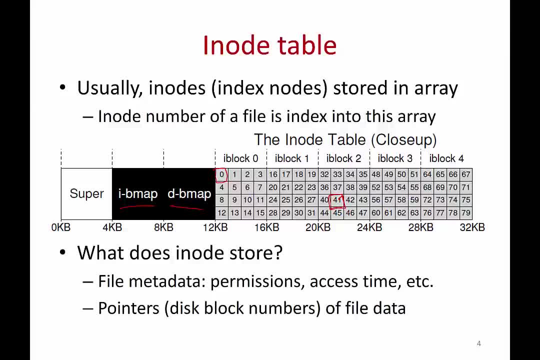 information about the specific file. so what information does it have? information does the I note store? it will store a whole bunch of metadata about the file, like who has permission to access the file, when was it last read, what is the size of the file, and so on. 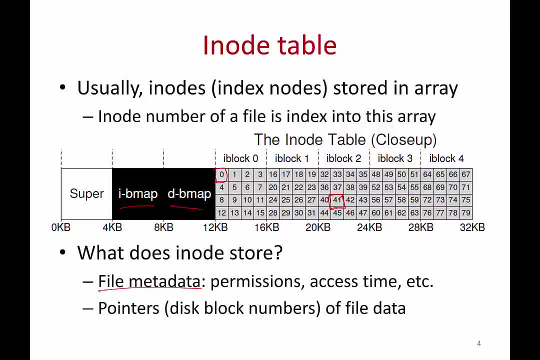 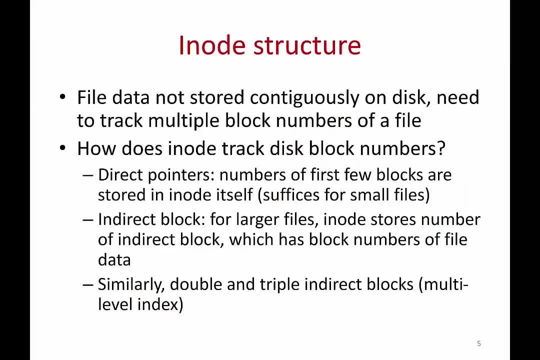 and then another very important thing that the inode stores is pointers to filed data, right? so note that in the data region the filed data need not be stored contiguously. there might be a block here, a block there, a block somewhere else, and the inode must basically store all the data that it has. 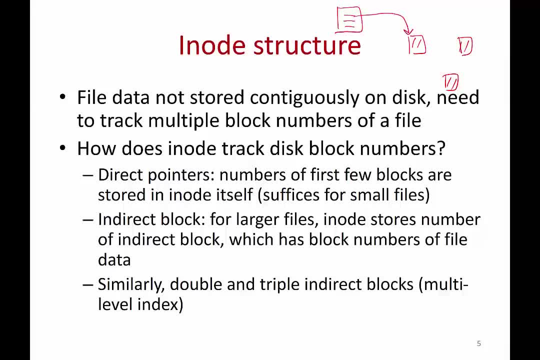 the numbers of all of these blocks. it must store pointers to all of these blocks right, so that the user knows where all the data of the file is located, right? so the most important function of an inode is to store pointers to all the data blocks of the file, right? so of course you, if 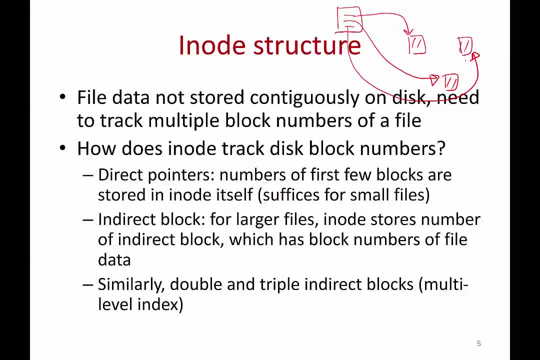 the file is really large, you might have a lot of blocks. you cannot store all of those pointers in one inode, right? so the way inodes are typically structured is like a multi-level index. what does that mean? the first few blocks of a file: you directly store their block numbers in the inode. 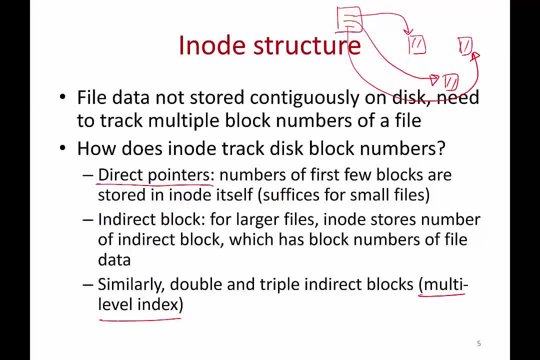 these are called direct pointers, and if your file size is small, maybe you have space for 10, 12 block numbers. you directly store them in the inode, and for more small files this is enough. but if your file is larger than this- the number of block numbers that can be stored in an inode- what do? 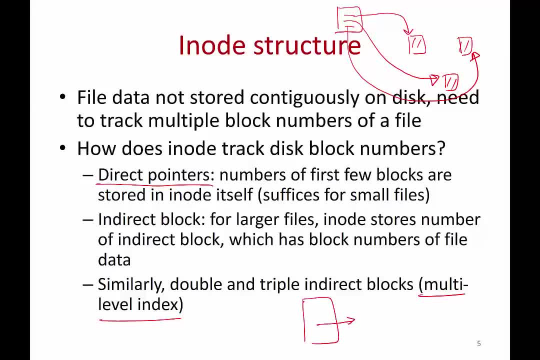 you do, the inode will basically store all of the pointers that you have stored in the inode, and then you can also store the block number of a block, which in turn has pointers to all the data blocks. right, this is called a indirect block, and if this is also not enough, then the inode will. 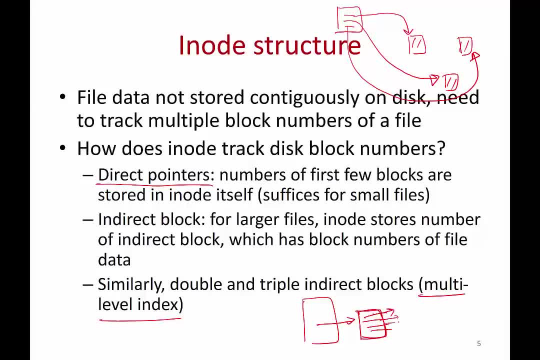 store the block number of a block which stores the block numbers of a few other blocks, which in turn will store block numbers of the file data. right, so you can have several indirect blocks. you can have a double indirect block, a triple indirect block, and so on until the entire file. 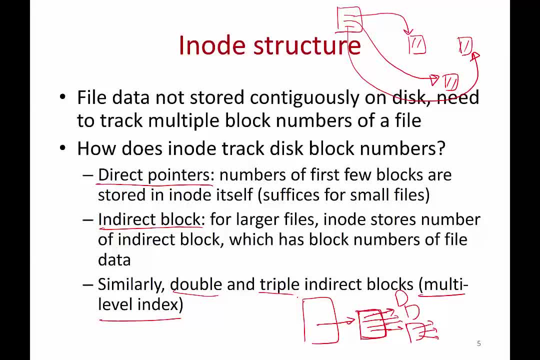 size can be accommodated, right, given the number of block numbers you have to store for a file you might want to. the direct pointers might be enough, or you might need a single indirect block, or a double or a triple indirect block, and so on. right, so this is called a multi-level index. 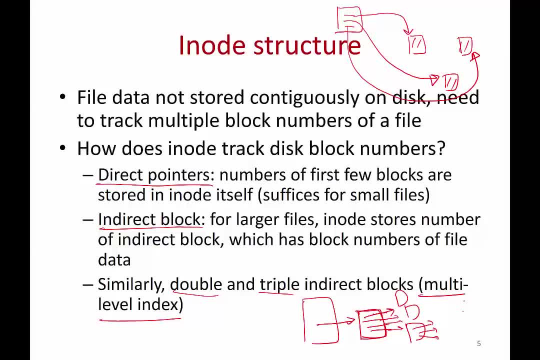 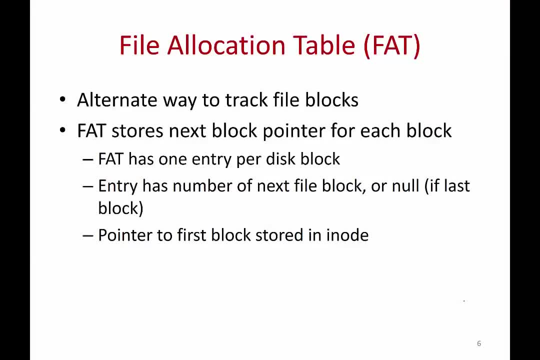 and this is a common way in which an inode is created. this is the common structure of an inode in modern operating systems. there's also an alternative, this which is called a file allocation table or a fat right. there's an alternative way to track all the blocks of a file instead of storing. 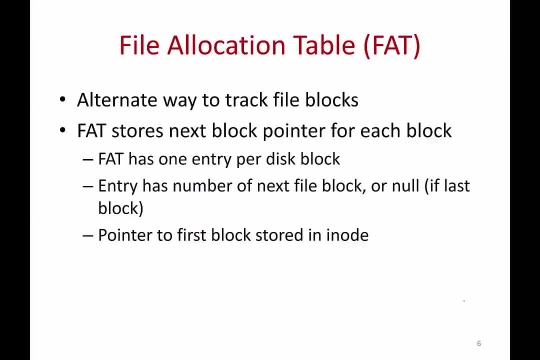 them in a multi-level index in an inode right. so this was used in some of the older windows operating systems. so what does the fat container? fat contains one entry per block in the file system and that entry points to the next block of the file or it is a null pointer right if it's the last block of a file. 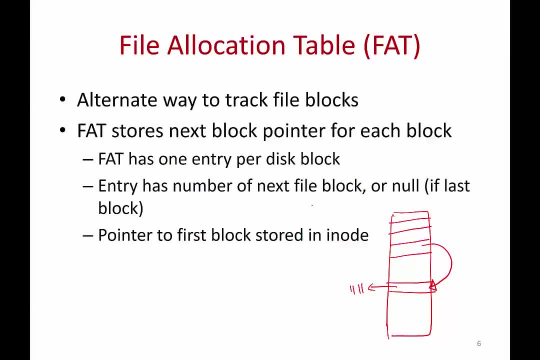 right. so if your file has three blocks, then you only remember the block number of the first block of the file, and that first block will store the number of the second block, and the second block will store the number of the third block, and so on. right, and the last block will simply point to null. 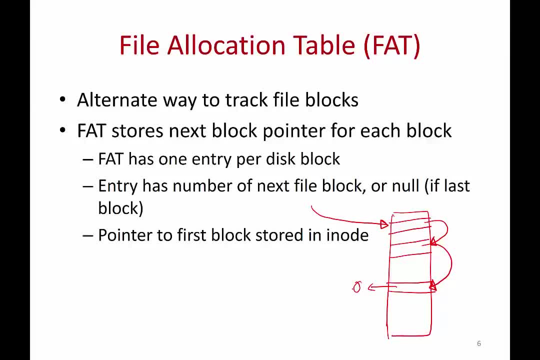 so this is a file allocation table. so in a file allocation table you have one entry per disk block and you just remember the first block number and all other block numbers can be got by following the pointers in the file allocation table. so this is an alternative way to track all the data blocks of. 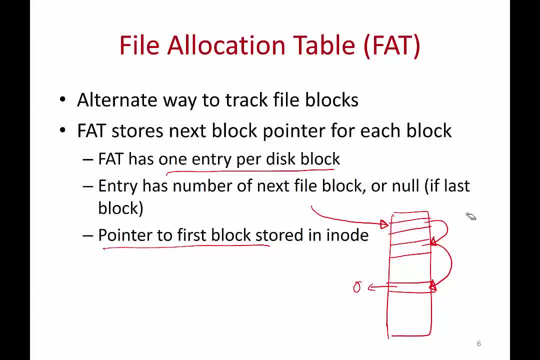 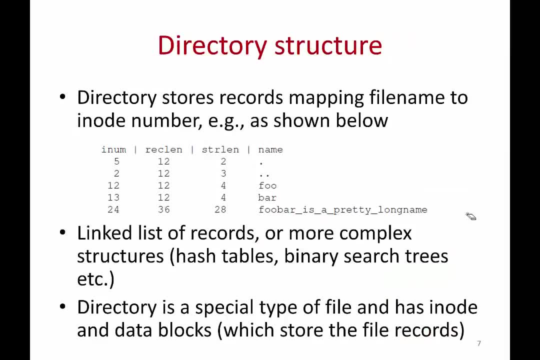 a file, but the more common one today is to use an inode which stores direct and indirect pointers to all the block numbers. so that was about it for this video about files, the data structures related to files, which is the inode, And next we go on to the directory. So what is a directory? A directory is simply a mapping from file name to inode number, right? So, for example, a simple directory could store information like this: it could store the inode number and it could store the file name and some string length of the file name. So here the directory probably allocates records in multiples of 12.. So for small file, 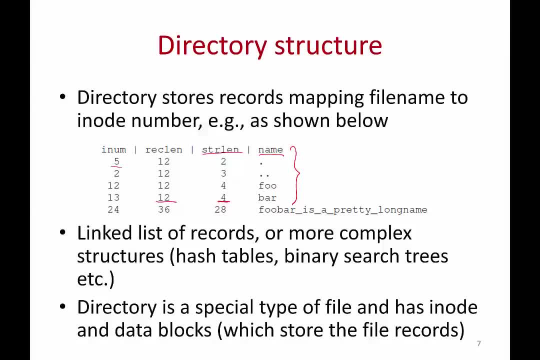 names. you have a record of length 12.. And then string length here indicates that the file name is three characters plus a null character. that is four. right For longer file names. you might have longer records and so on. So basically you have the file name and the inode number And these can be maintained in any structure. different file systems have different structures. For example, you can simply store them all as a linked list of records. you can use hash tables. you can use binary search trees. 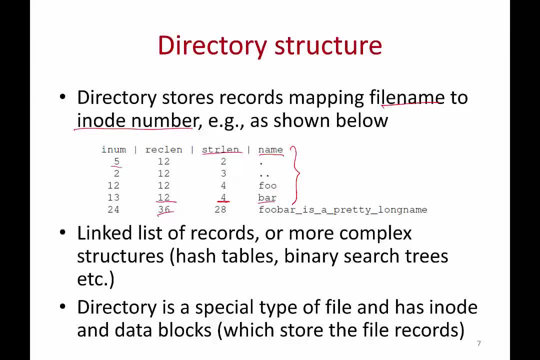 right, You can organize this file name to inode number mapping in many different data structures, right? And all of this content, right? This linked list of records and all of this information is simply stored as a file on disk. So a directory is simply a special type of a file. It also has an inode number, right? So there is an inode for a directory that tracks all the data blocks of the directory and 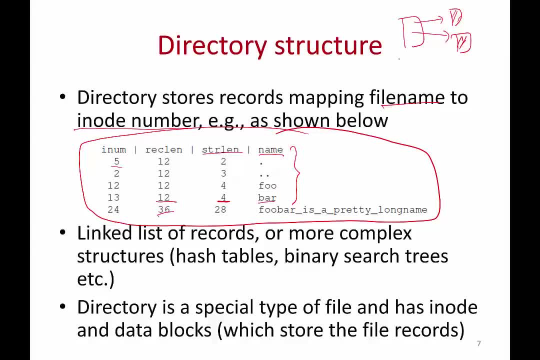 these data blocks store all of these records, right? These data blocks, this is the inode and this is the data blocks, And these data blocks store all of these linked lists or any other data structure of records of the file. So directory is simply a special type of file whose contents are the file names and inode numbers of the files it contains. 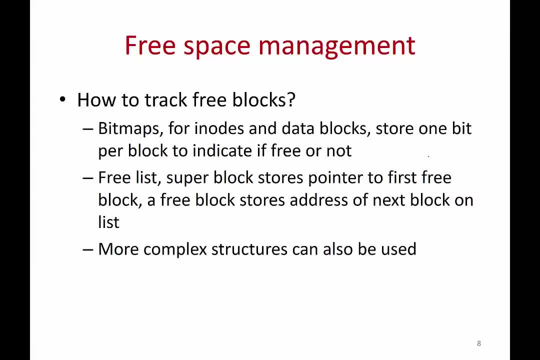 So the next question that comes up is: how do you track all the free blocks? right, So, the blocks that store the inodes, the. so the next question that comes up is: how do you track all the free blocks? right, So, the blocks that store the inodes, the block that stores the inodes, the file lockers and so on And so on. So directory is a special type of file and all of these records are useful to수뽁. 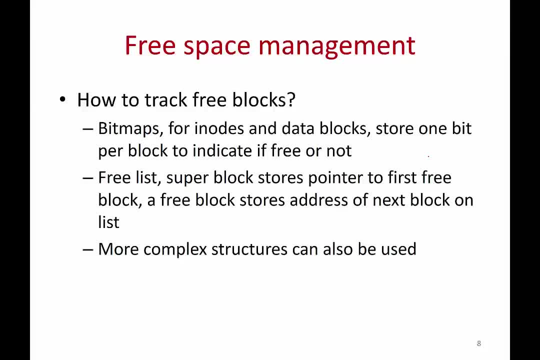 of records are useful. toמןade you to사 who pendert me Ek-财 1515 deeds inside. I want a name. their keeps up as per quase out. blocks that store file data. there might be a lot of free blocks in there. some blocks might be used. 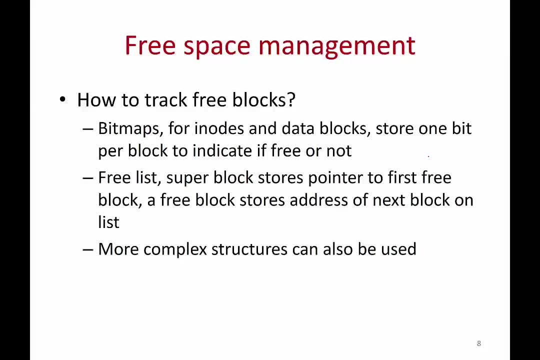 some blocks might be free. how do you track all of this? so we've seen one simple idea is a bitmap. what is a bitmap? you have one bit for every block and that bit is one. if the block is occupied, it is zero. if it is free, right. so you scan through the bitmap once you find a zero entry, you know. 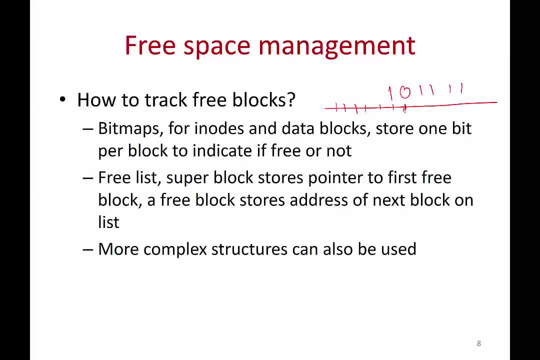 that if the 15th entry of the bitmap, if the 15th bit, is zero, then the 15th block is free. let me go ahead and use it. right? those are bitmaps, or you can also have a free list, right? so your super block stores a pointer to the first free block and inside this free block you store the number. 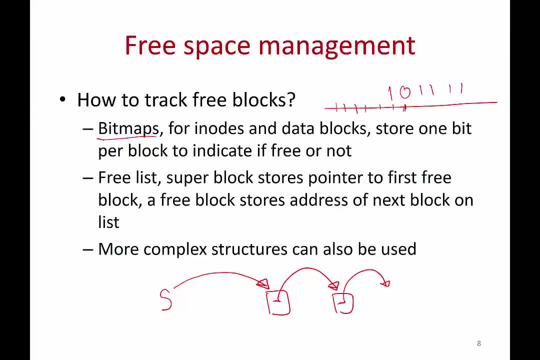 of the next free block and inside that free block you store the number of the next free block, and so on. you can also maintain a link list of free blocks and of course you can also have any other kind of data structure to track the list of free blocks in a file system. 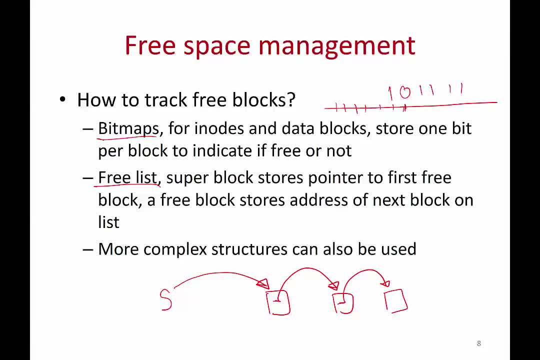 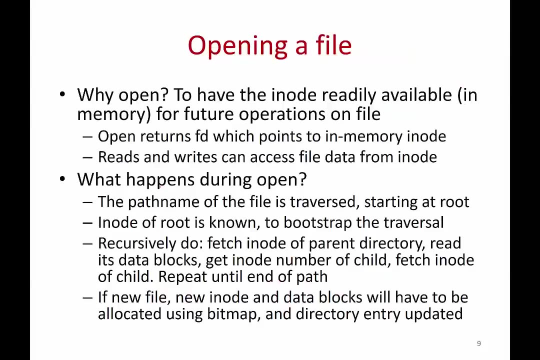 so I hope that you found something, michael combine. so note that these are all the design choices that different file systems make: how to structure the directory, how to track the data blocks of a file in an inode, how to manage three blocks right. different file systems make a different choices here. so, given all of these data structures, let's see how do you do operations. 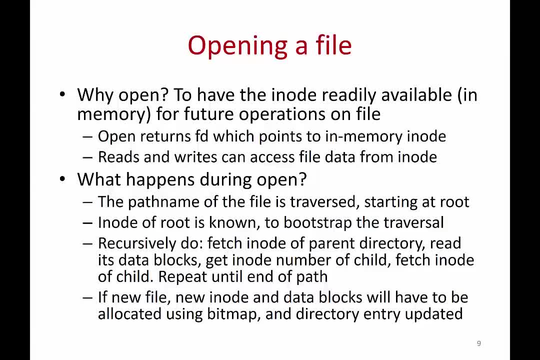 on a file. how do you open a file? now did 8 from a file and so on. right so far, some all. why do you have to open a file? open system call is to make the inode readily available any time I want to read or write from. 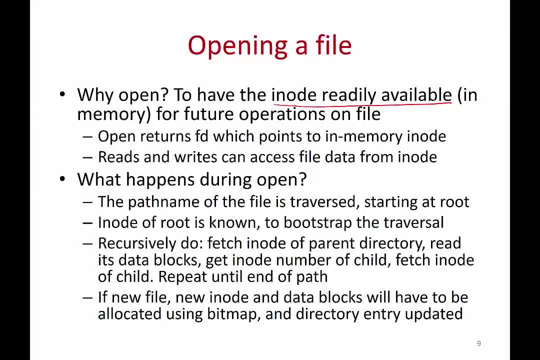 a file. I should have the inode of a file readily available so that the inode has pointer to all the data blocks and all other information about a file. so this inode, I want to get it into memory from disk. that is the purpose of the open system call and the open system call returns a file. 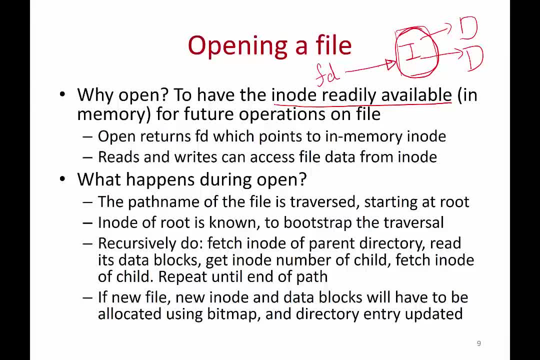 descriptor which simply points to this inode in memory. given the file descriptor, you can get to the inode in memory- we'll see how in a little bit right, so that in all future operations on a file, like reading and writing, you can simply easily access the inode, easily access the data. 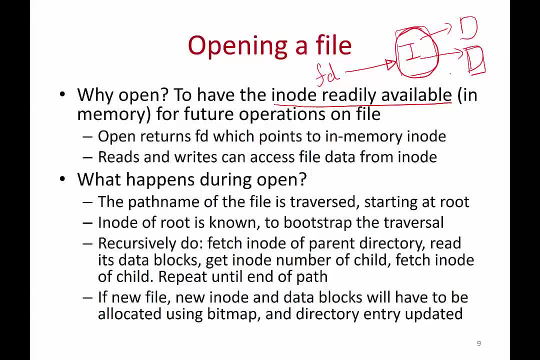 block and tell the disk: hey, get me this data block and that data block, right. so now what happens during open? the goal of open is to locate the inode of a file. what? how do you find the inode of a file? you try to locate the inode of a file. and you try to locate the inode of a file. you try. 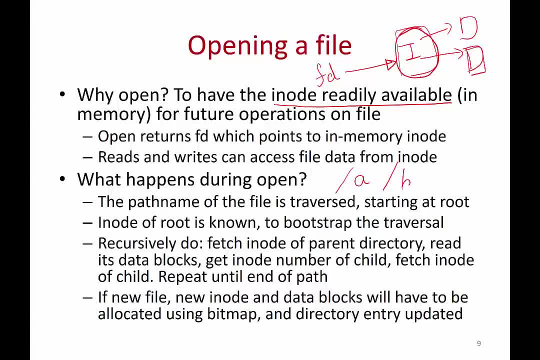 traverse the path name. suppose you have a path name like a slash a, slash b, slash c dot text. if this is your file, then what do you do? you start with the root inode, right? you start with the root. so you know the inode number of the root. you go fetch the inode of the root. 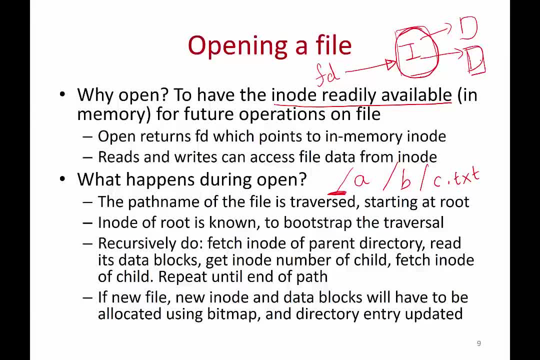 then, from the inode of a root, you fetch the data block right. anytime you fetch the inode of a parent directory, what do you do? you read the data block of the root in order to get the inode number of the next component in your path. so i get the inode of the root, i get the data block of the. 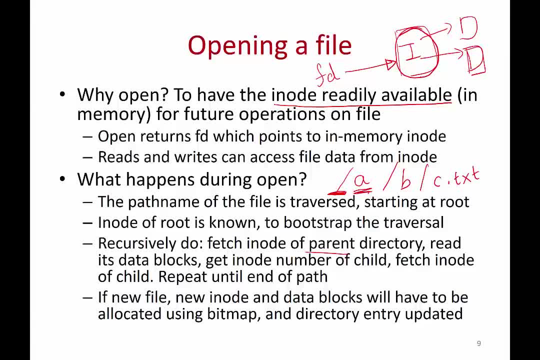 root. inside that data i search for the file a. then i get the inode number of a. then i get the data block of a. inside that i search for the file name b. now i've gotten the inode number of directory b. then from the inode number i know the inode number of the next component in your path. 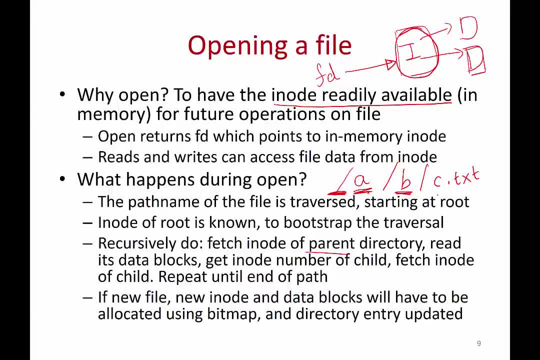 know where all the data blocks of b are located. i go get those data blocks and in those data blocks i search for the file c dot text. and once i locate that file name, i get that inode number and then, given that inode number, i'll go fetch the inode of c. right, so you recursively walk down the path. 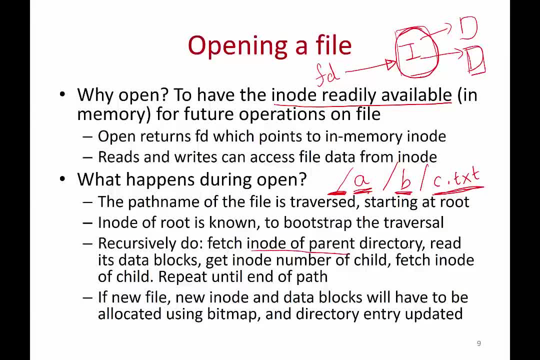 go from the inode of a parent to the data block of the parent, to the inode of the child, and so on until you hit the final file name. and once you've gotten the final, you've located the entry of the file name, you get its inode number. 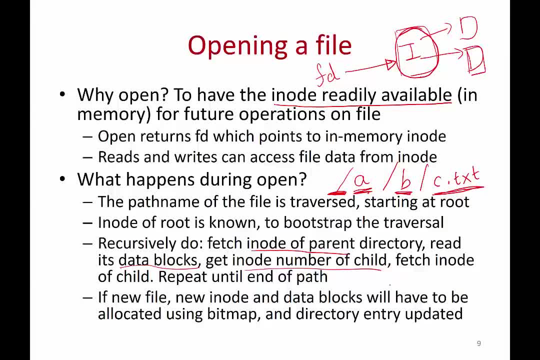 then you copy that inode number from disk into memory right. and if this file does not exist, if you're creating a new file during open, then what do you do? you will allocate a new inode and you will allocate new data blocks using the bitmaps. you know which inodes are free if the c dot text. 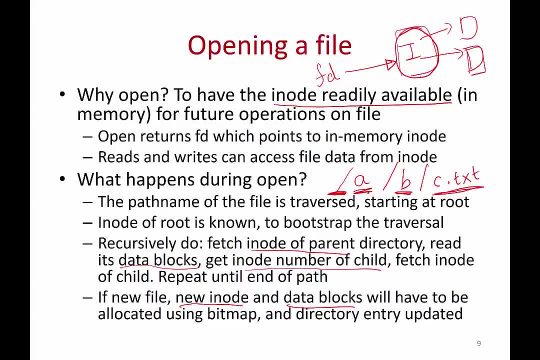 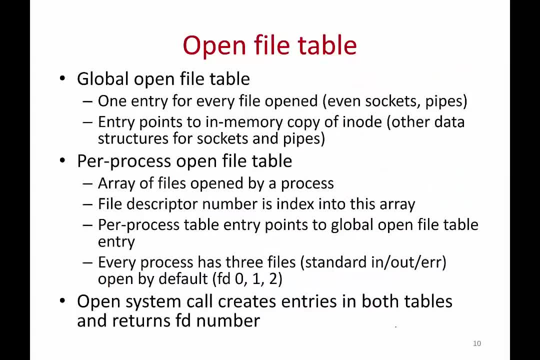 during open. so note that the kernel uses a set of data structures to track all the open files. that is called the open file table. right? so you have a global open file table which has one entry for every open file, right? note that this file table also stores things like sockets and pipes, and 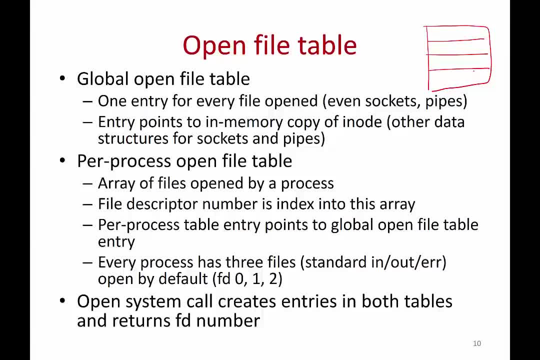 all of that right, but let's ignore that for the moment. so every time you open a file, an entry is created in this open file table, and this entry points to the inode of the file, right and then. so this is the global file table, and then, for every process, you have an array of all the files. 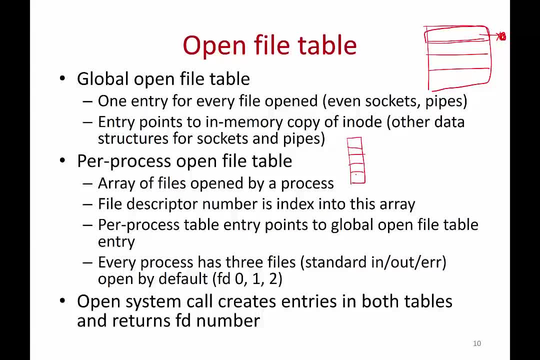 that the process has opened. so this is called the per process open file table, and a file descriptor that is returned is simply an index into this array, right? so if this is the fourth file that your process is creating is opening, then you will get an fd number of four that will be returned in. 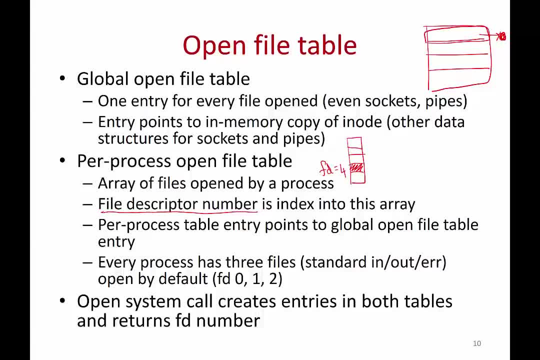 your open call. and this fourth entry in this per process open file table will point to some entry in the global file table, which in turn will point to the inode of the file right. so why do you need to read a global file table? simply because you know if multiple process is open the same file you can. 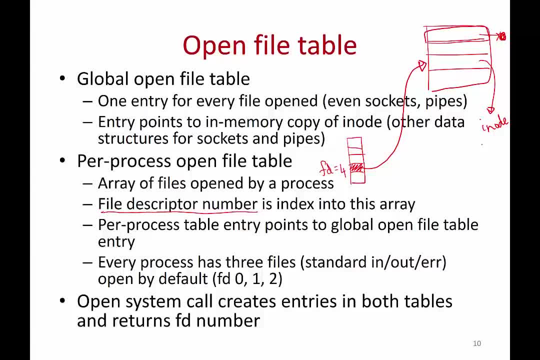 have one location where all the pointers to the inodes are stored. and again, a per process file table is simply for convenience, right? you can return the file descriptor numbers you can return to. a process can be starting from zero, one, two and so on, so every process has three files open by. 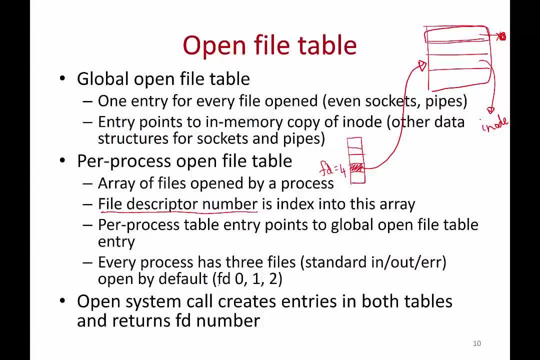 default, when the process starts, the operating system opens three files, which is file descriptor number zero, one, two which point to the standard input, standard input and also the file descriptor output and standard error, that is, the files opened to read from the screen and the keyboard and so on. so these are opened by default and when a file opens, 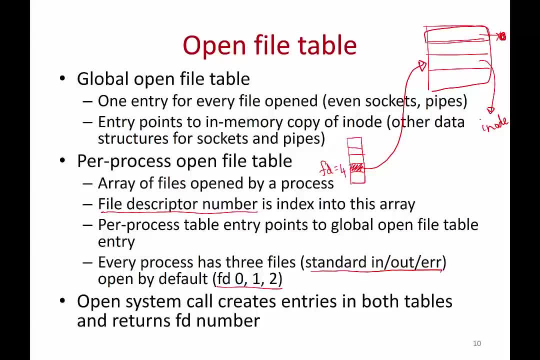 when a process opens other files, you get higher file descriptor numbers, starting from 3, 4, 5 and so on, right, and this file descriptor points to an entry in the global open file table, which in turn stores a pointer to the I know right. in the end, given a file descriptor, what can you do? the open system call returns the. 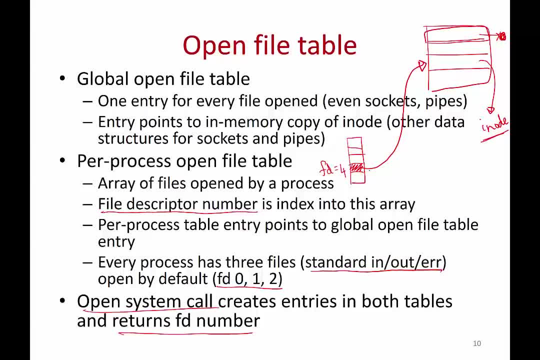 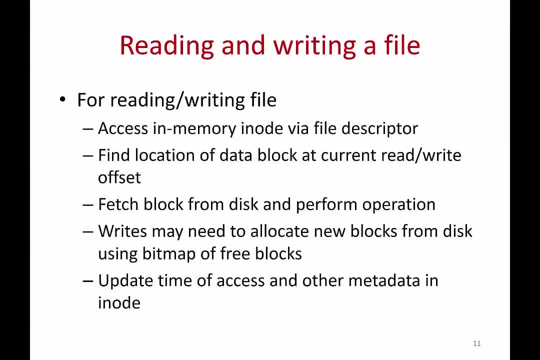 file descriptor, and from the file descriptor you can locate the I node of the file, right I node of an open file. so then, from now on, given that you have easy access to the I node of a file via the file descriptor, all other operations are fairly straightforward. if you want to read from a file, what do you do? you? 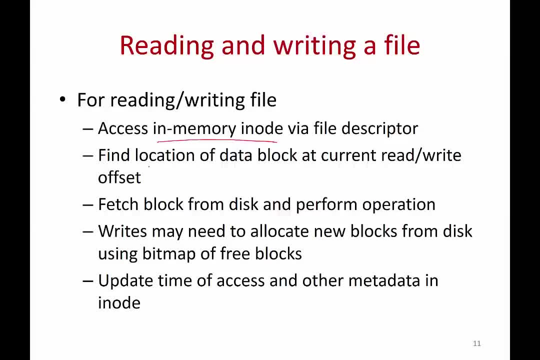 access the in-memory I node. the I node has locations of all the data blocks. then you fetch these data blocks from the disk. you tell the disk: give me block number 23, block number 84 and so on. how do you know these block numbers you get? you've gotten them from. 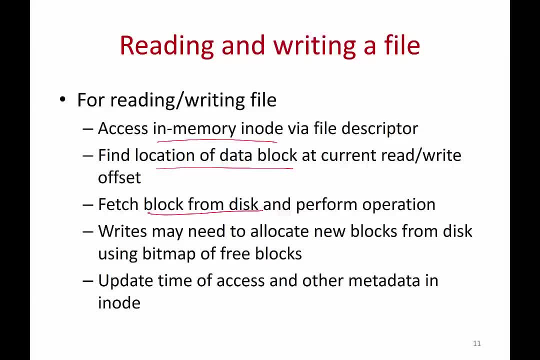 the I node and you fetch the blocks from this and if you are writing, then you make changes to these blocks and you give them back to the disk and so on. right, and if you have to allocate new blocks for a file- the file size is increasing. you have to allocate new blocks, then you go ahead. read the bitmap. 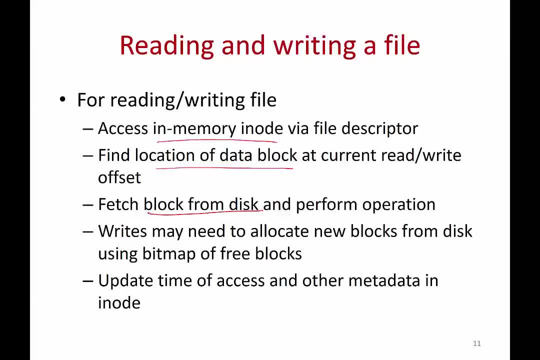 and you get a free block from the bitmap and you write to those new blocks. right and anytime you access a file, you will also access the I node, because you update our various metadata in the I node and so on. so any operation on a file usually touches multiple different blocks. you know the actual data blocks. 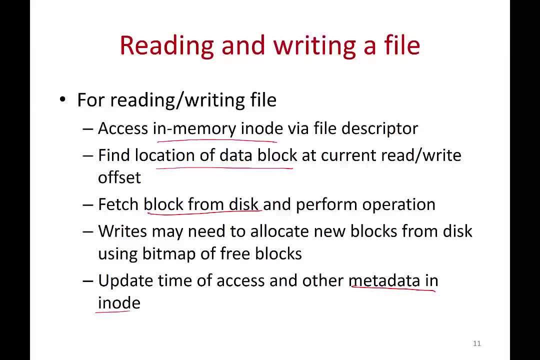 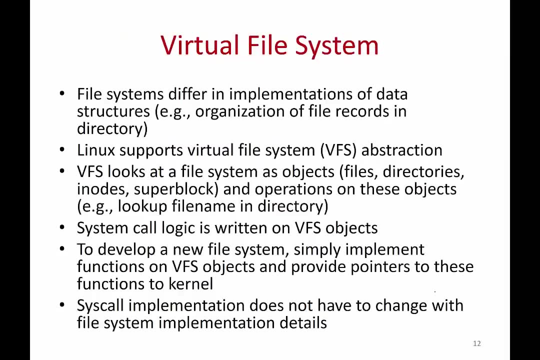 the metadata in the I node, the bitmaps. all of these things are touched when you do any operation on a file. so the key takes away here is any file operation, will you know, require multiple accesses to the disk right. so the operating system has several optimizations in place to handle. 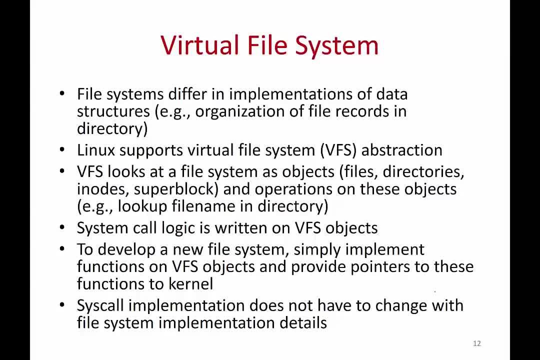 all of this complexity, right? the first optimization, or rather abstraction, is that of a virtual file system, right? so we've seen that different file systems differ in the implementation of all the data structures and so on. right, one file system might store directories and so on, but in the implementation of all the data structures and so on, right, one file system might store directory. 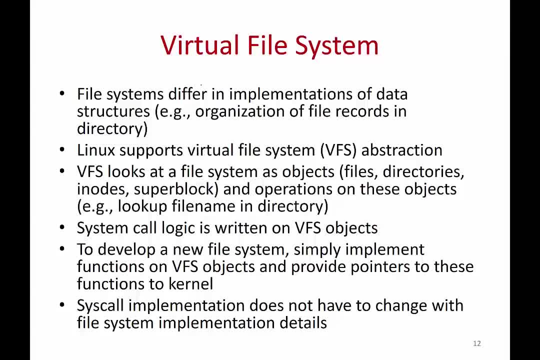 in a link list, another file system might store it in a search binary, search tree, and so on. so does this mean that the implementation of the system calls also has to change with different data structures? well, that doesn't have to be the case, right? so what Linux does is it provides an 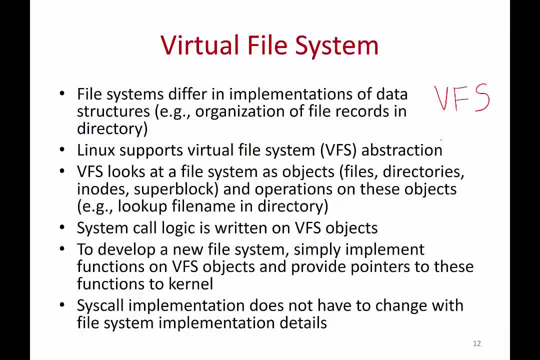 abstraction layer. it provides a system called the virtual file system or VFS. so any system calls that the application makes right. the code for the system calls is written in terms of at a higher layer of abstraction. for example, the VF looks at a file system as a set of objects. you know there's files. 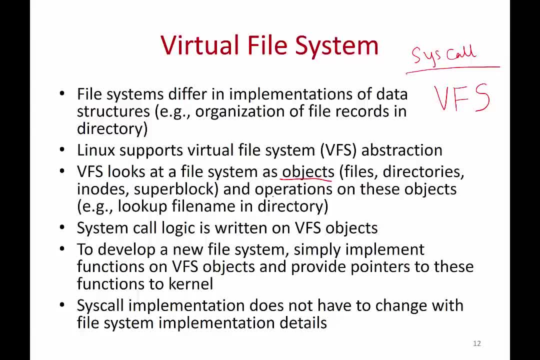 there's directories, design nodes, the super blocks and operations on these objects. for example, on a directory you look up a file name right and an I node, you might add a data block. you might read the data block. so all these are operations on these objects. so when you write system call logic in Linux you 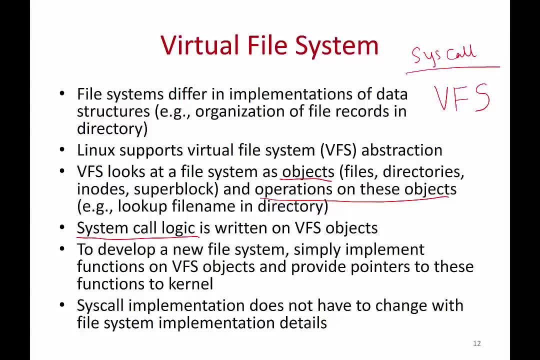 will only write it in terms of these objects. so if you want to open a file, you will say: read the root I node locate. look up this file name in this I node in this directory, look up the next file name in the next directory, and so on. 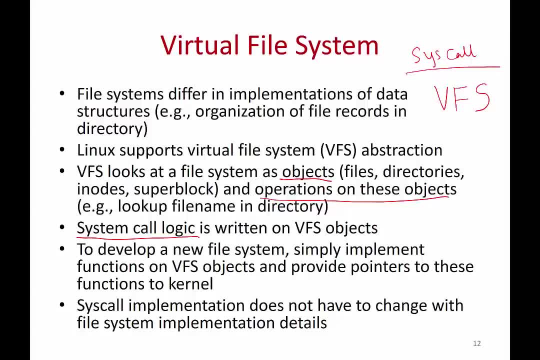 you're going to write all your logic for system calls in terms of these VFS objects and the implementation of a file system will simply implement these objects and these operations, right? if you want to implement a new file system, you create data structures for all of these VFS objects. you have a way to implement all of these operations like look. 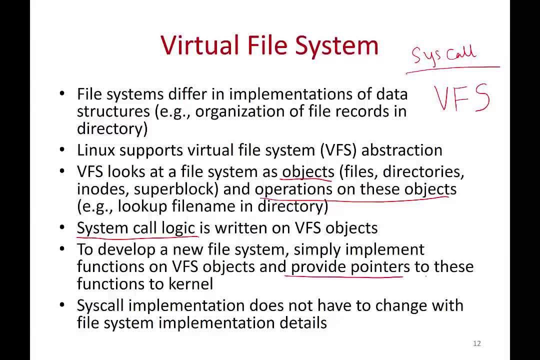 up and so on on these objects and you provide pointers to all of these functions, to the operating system. so if you're developing a new file system, you do not have to rewrite the entire system call logic. all you have to do is support these objects and these operations and the system. 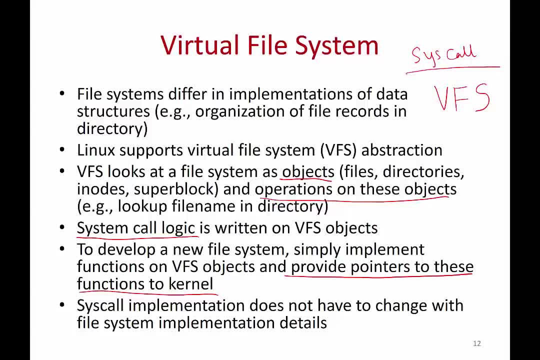 call logic can be reused. it is already written in terms of VFS objects, right? so this is one way in which modern operating systems cope with the huge complexity of a large number of file systems. the system call logic just writes on is written in terms of VFS objects and the underlying file. 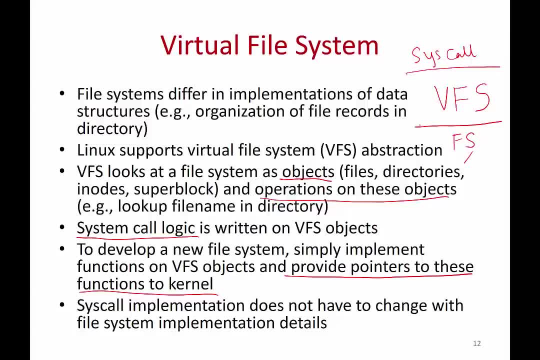 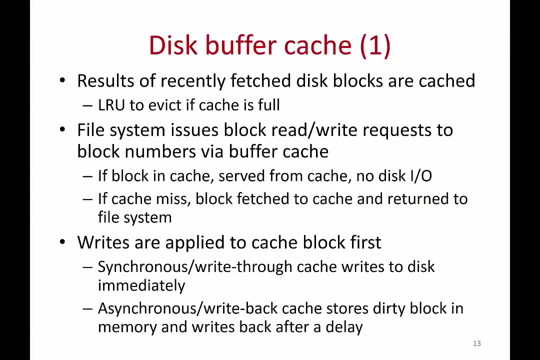 system provides all the code for the VFS objects as well as the operations on the object right and provides pointers to these, so that when the system call logic has to call some operation on a directory, the corresponding function in the file system is invoked. and the other idea that operating systems use is that of 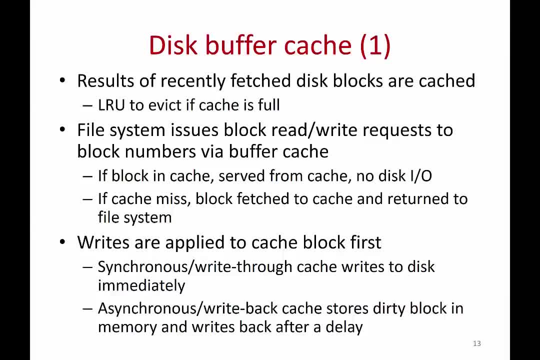 this buffer cache. as we've seen, every operation of a file will require reading and writing to multiple disk blocks. so what the operating system does is the recently fetched disk blocks will be cached, right. so block number 23, block number 84, what that have been recently read. 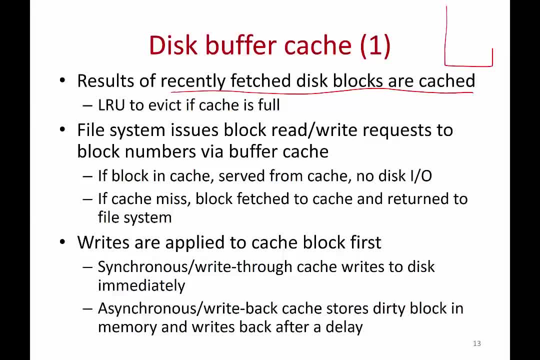 from the disk. they will all be stored in a cache right and this cache has a whole bunch of recently read blocks and if the cache gets full you're going to evict it. use some policy like LRU to evict the cache when it's full right and whenever a file system says read a certain block right. 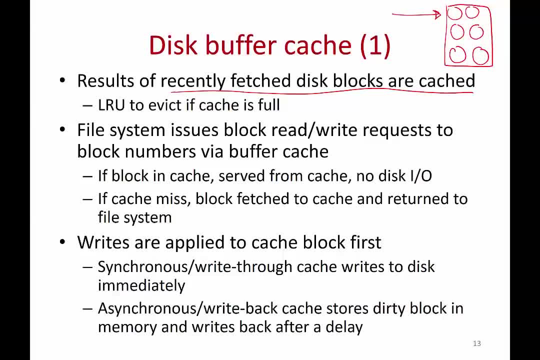 the buffer cache first checks in the cache. if the file is there in the cache, it will return it directly from the cache. there's no need for a disk IO, and only if there is a cache miss. if the particular block has not been recently used, it's not there in the cache. only then will you. 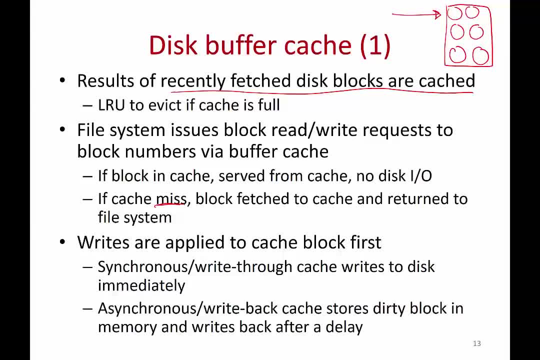 go to the disk. right, you will do a disk IO, you will store a copy in the cache and return it to the file system. and similarly this is for read operations. right, if you're trying to read, you first read in the cache. only in a cache miss, you read from the disk. and in the case of writes also, 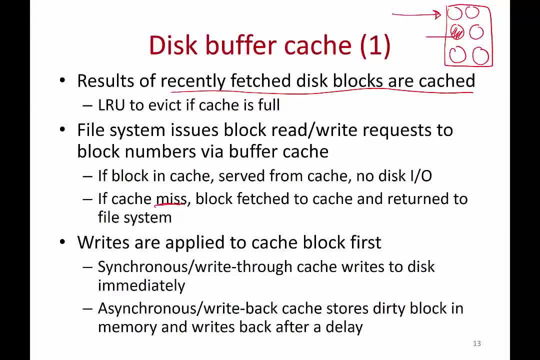 you will first write into the disk block and then at a later point of time you're going to push that write into the disk, right? so here is a disk block in the buffer cache. you're going to first write to it and then at a later point this write is going to be pushed into the disk. so there are. 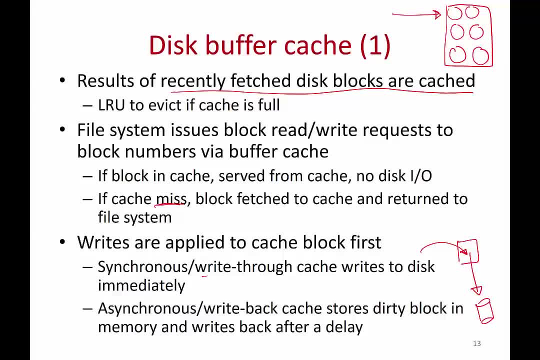 two types of buffer cache implementations. there's the what is called a sync runners, or a write through cache: as soon as you write into the cache, it will write to the disk immediately. and there's also the asynchronous cache, or a write back cache, which basically stores all of this dirty blocks in the cache and then at a later point of time when the disk is free. 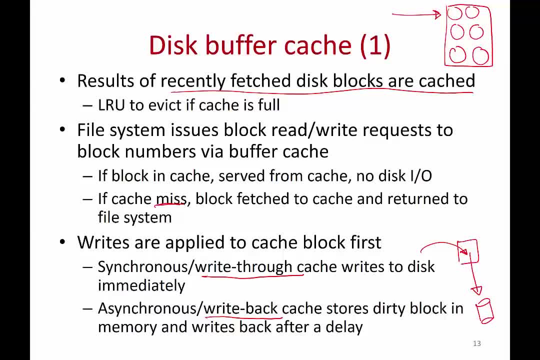 or when the system is free, it will go ahead and write back to the disk after a delay, right, so there, these are the two different flavors of implementation of the buffer cache. so the file system, of course, does not have to be aware of all of this, so you can just go ahead and write to the 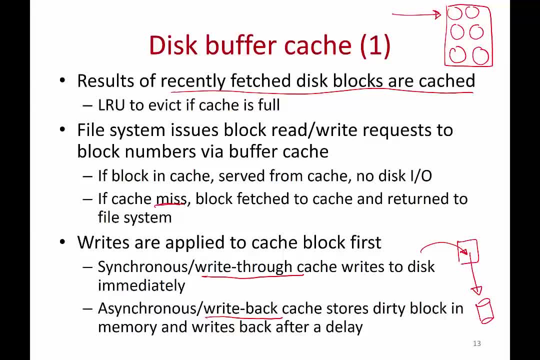 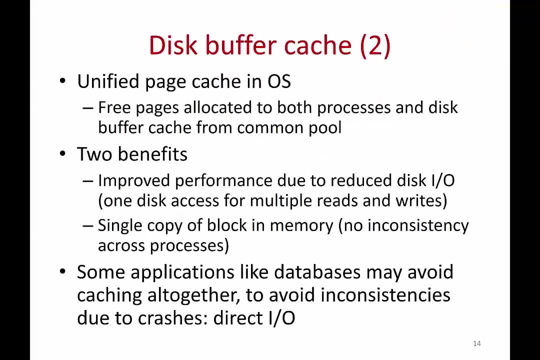 cache and then the buffer cache will do all of these details. the file system will simply say: read this block or write that block, and the buffer cache handles this complexity. so how much of memory is allocated to the buffer cache? usually this is a dynamic allocation right, whatever. 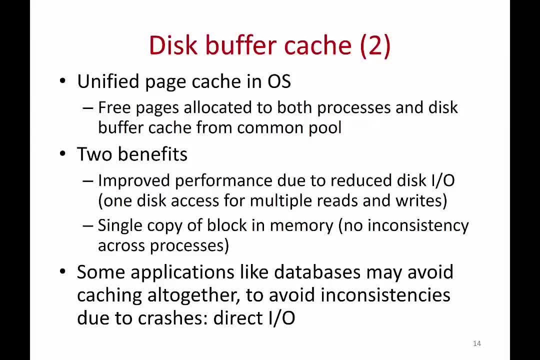 memory is free in your system that's not used by the other processes. a large chunk of it is given to the buffer cache so that you can improve performance, and the main benefits of using a buffer cache is, of course, obviously improved performance, right? so if multiple processes are, 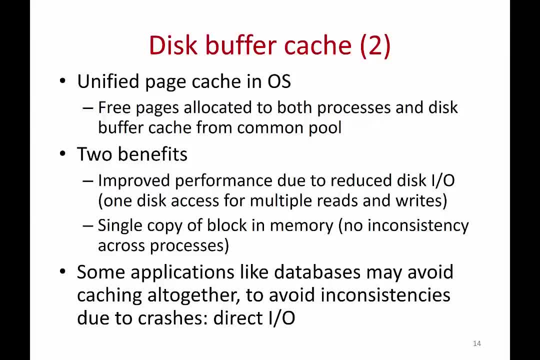 read the same block from the disk, then you will only go to the disk once and all other future reads will simply be satisfied by the cache. so certain important blocks, like you know the kernel code, or you know the inodes of the root directory, or the important directories or some hot files, 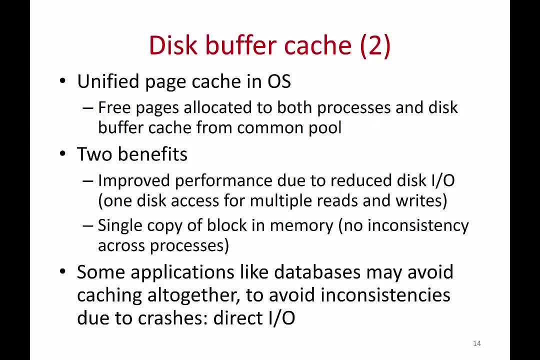 hot directories that are constantly being accessed. all of this are usually going to be found in the buffer cache and you don't have to go to the disk, so this improves performance. similarly for writes, if multiple processes are writing to the same block, all the rights are merged. 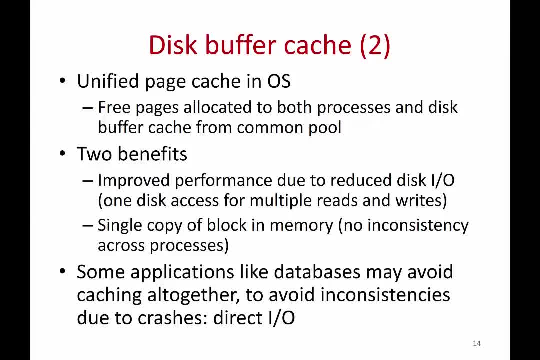 and you'll only go to the disk once. right. especially in the case of a write back cache which doesn't go to the disk immediately, multiple rights are clubbed before you go to the disk. this greatly improves performance of your system calls and therefore of the application. 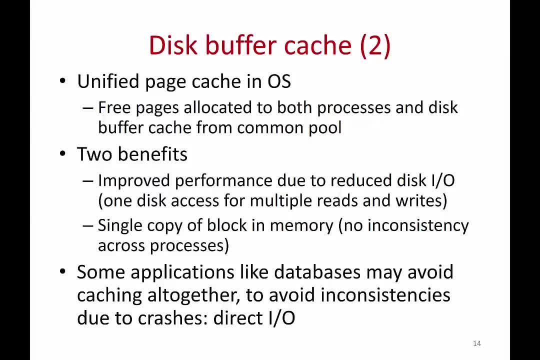 and the other sort of corollary benefit of the buffer cache is you only have a single copy of a block in memory. so if multiple processes are writing to the same disk block, you only have a single copy. therefore, all of those, all of their changes, will be merged you. 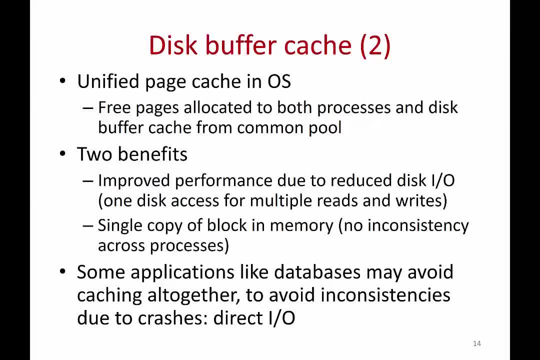 don't have two different copies of a disk block in memory ever, because the disk buffer cache provides a manages the synchronization, though of course the buffer cache is not always good and some applications may choose to simply avoid caching altogether. right, because the buffer cache might impose a certain amount of- uh inconsistencies in the might cause inconsistencies. 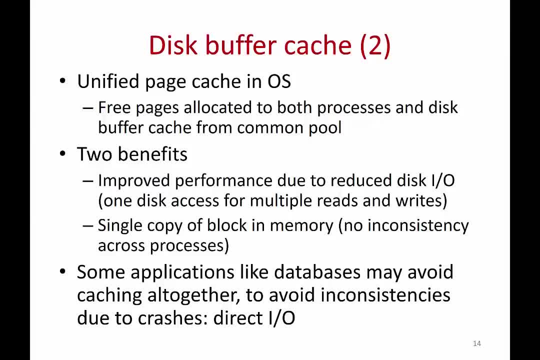 in the case of a crash, for example, the write has been written but it is still in the cache. it has not gone to the disk, but the application thinks it has gone to the disk. so all sorts of issues can happen and similarly the application also might want to do its caching itself. therefore certain 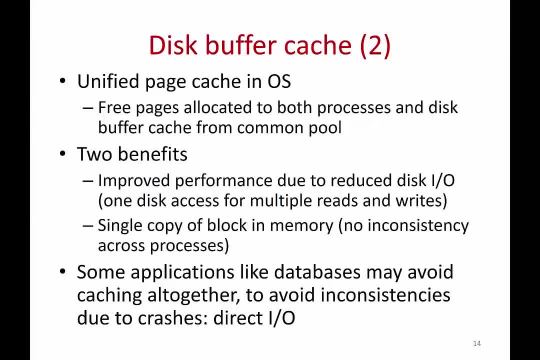 applications might choose to simply avoid the buffer cache altogether and do a direct io to the disk.